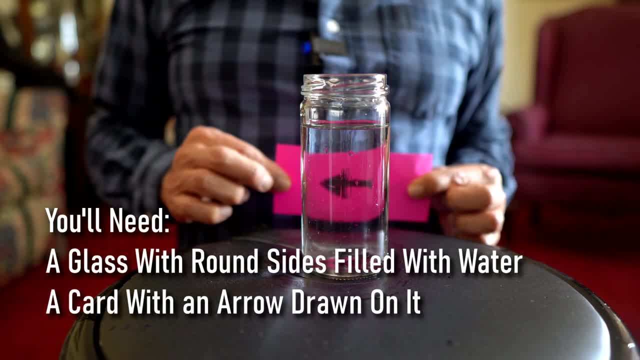 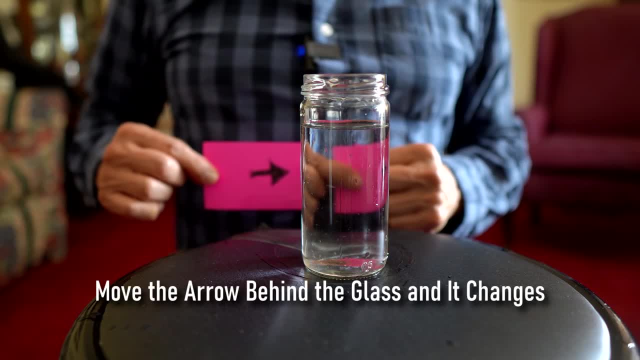 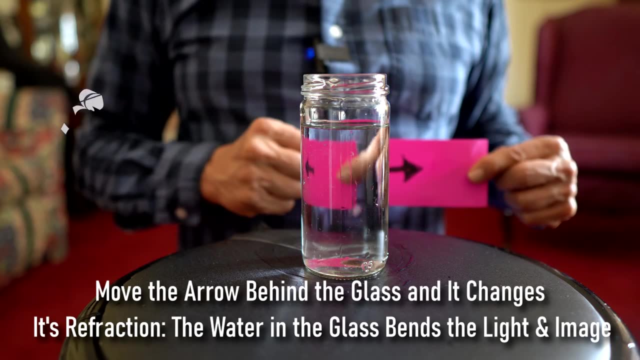 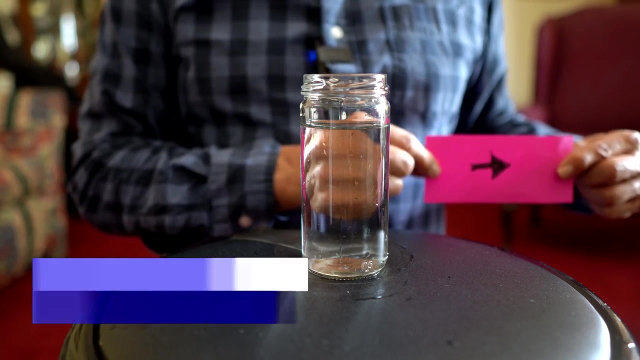 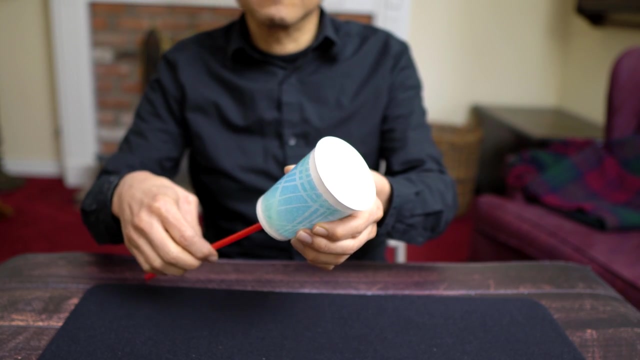 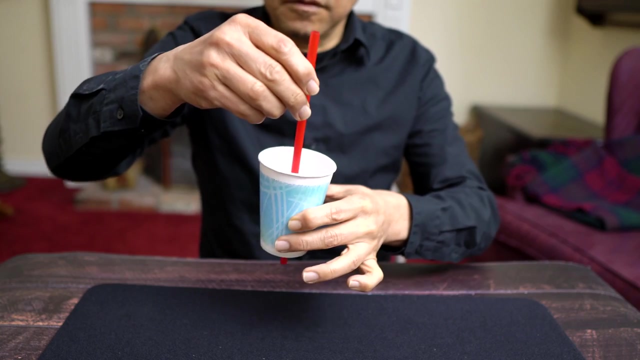 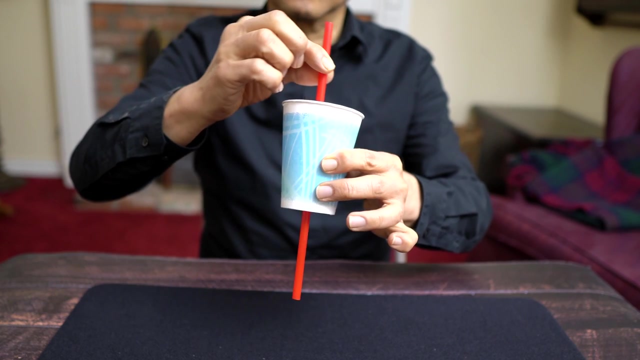 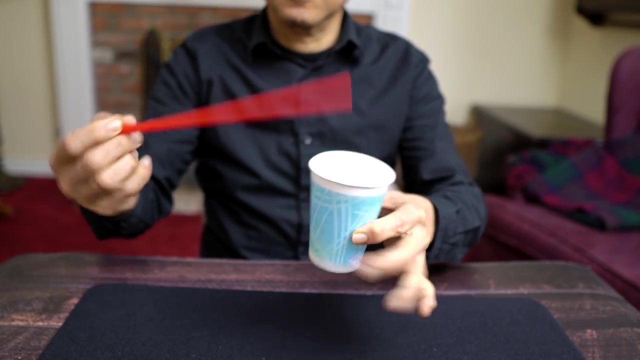 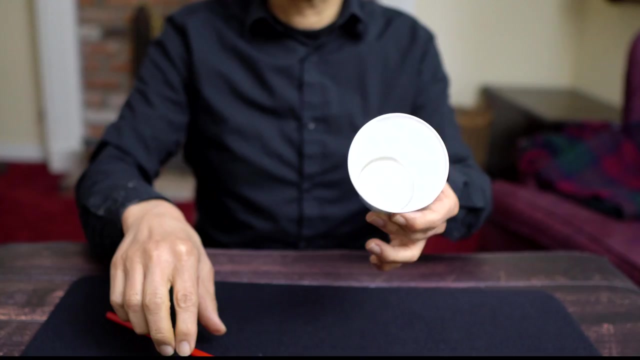 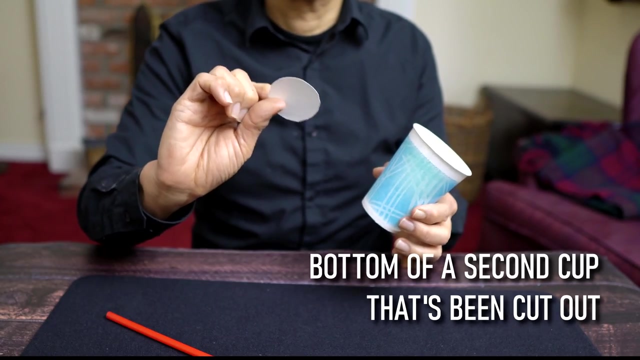 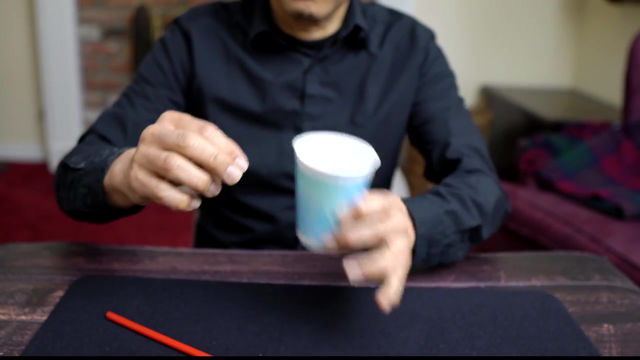 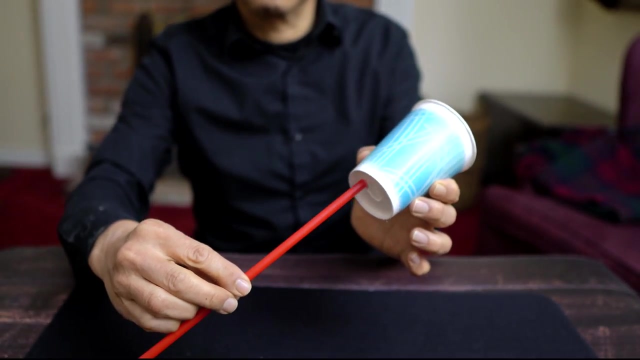 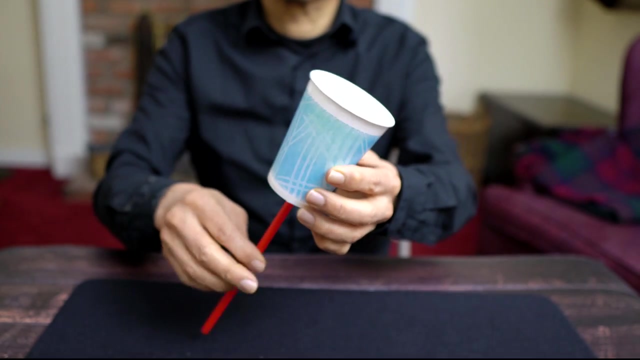 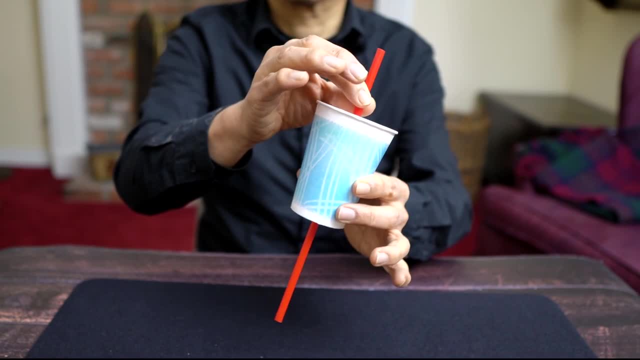 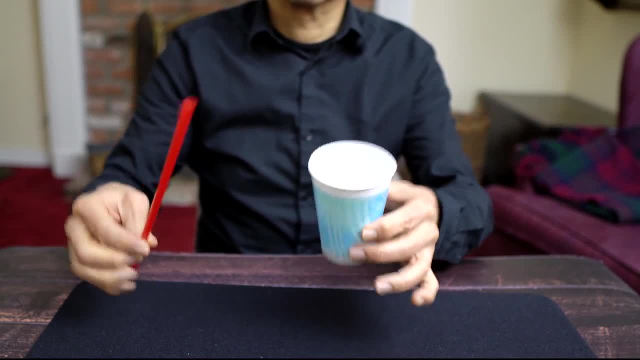 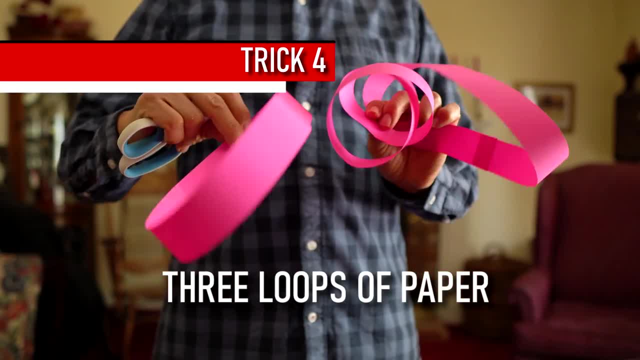 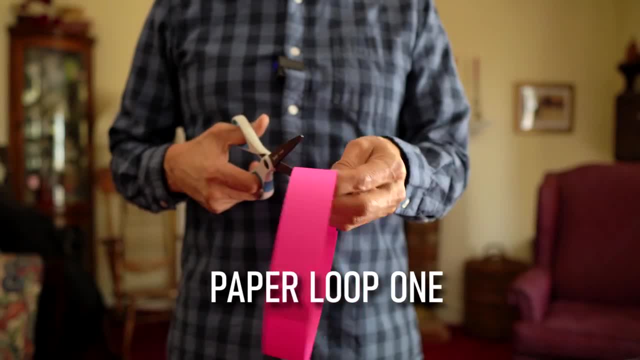 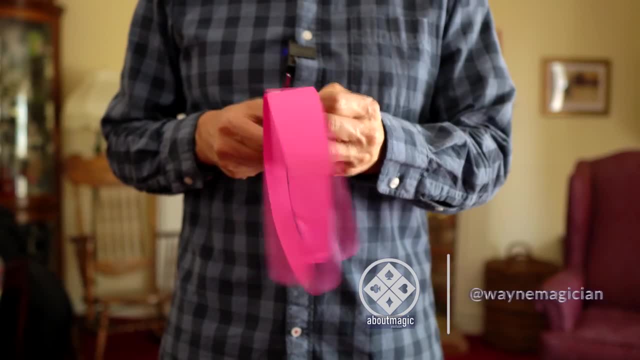 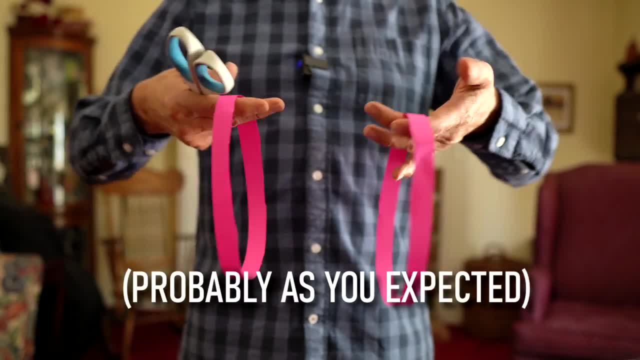 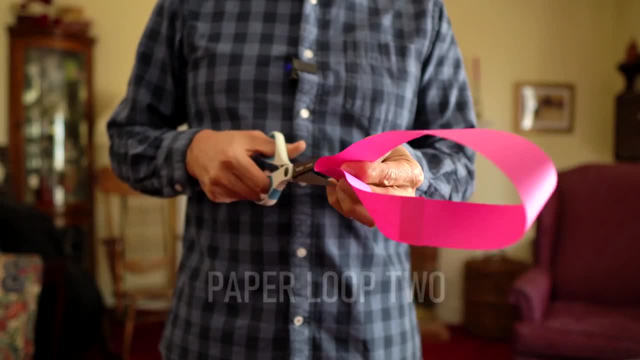 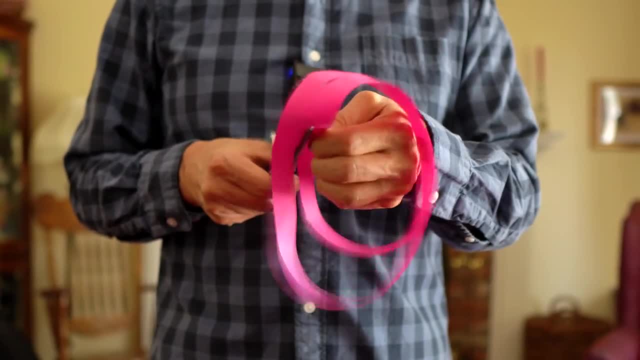 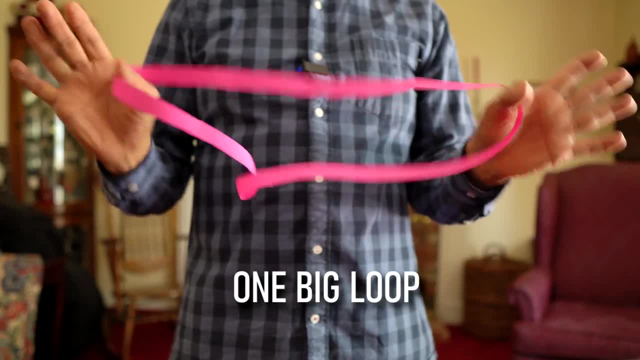 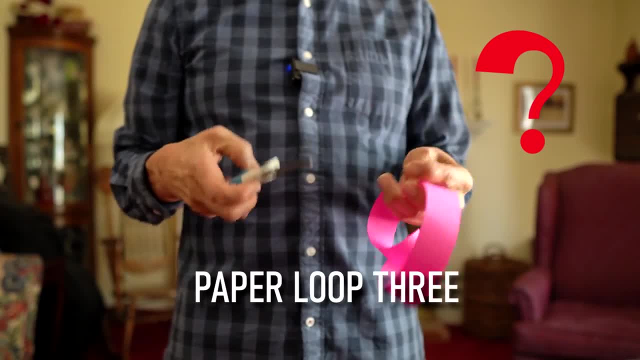 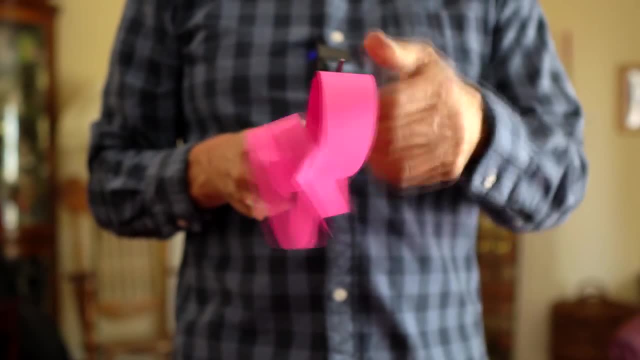 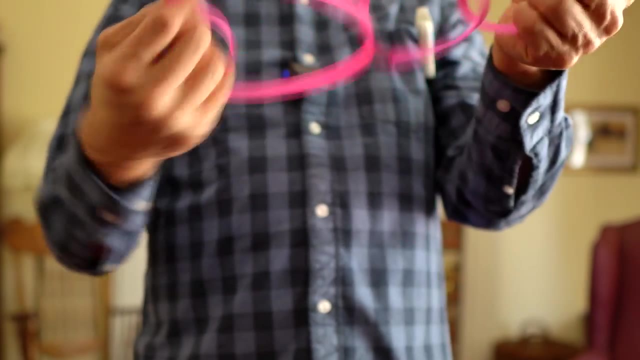 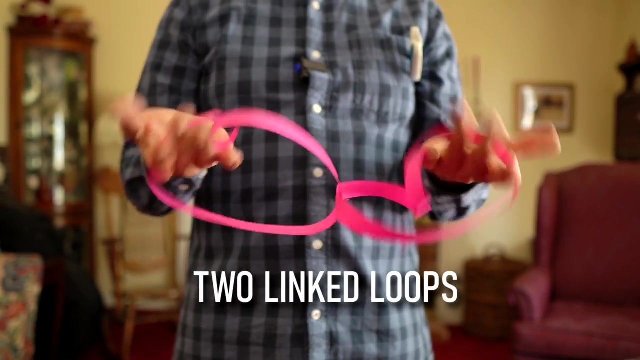 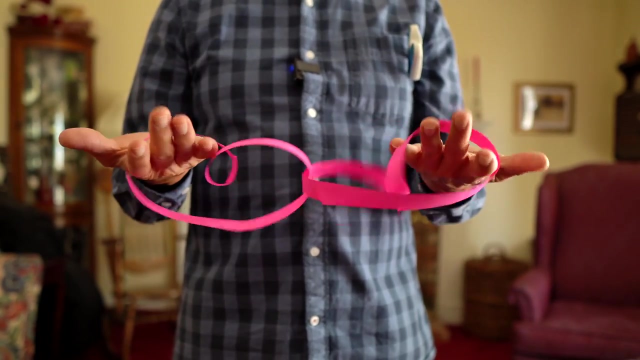 Amaze your friends with these easy magic tricks. Check them out. Amaze your friends with these easy magic tricks. Check them out. Amaze your friends with these easy magic tricks. Check them out. And we get two interlinked rings In this trick. there are three variations on the loops that you create. 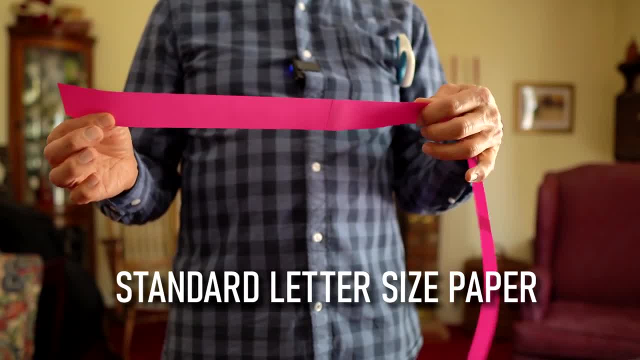 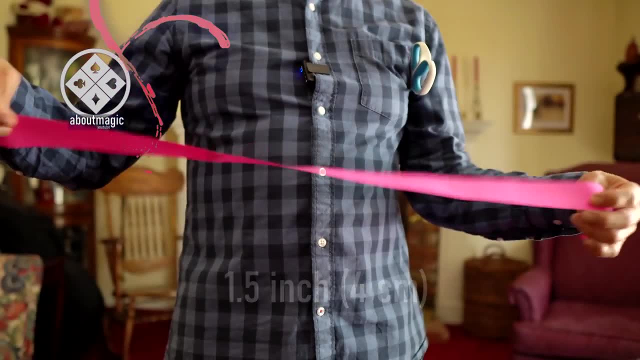 All I've done here is: taken an 8.5 by 11 sheet of paper, cut 1.5 inch strips lengthwise and glued them together right here, And then at some point I'm going to glue them together to make the loops. 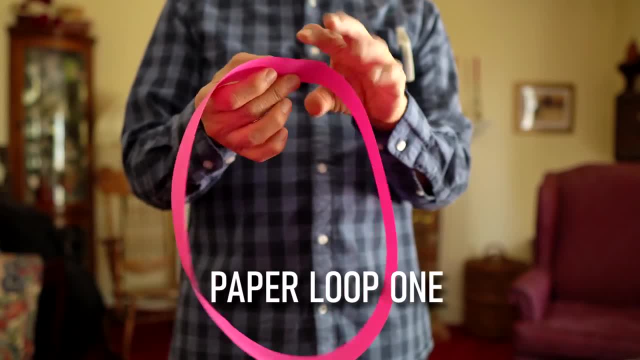 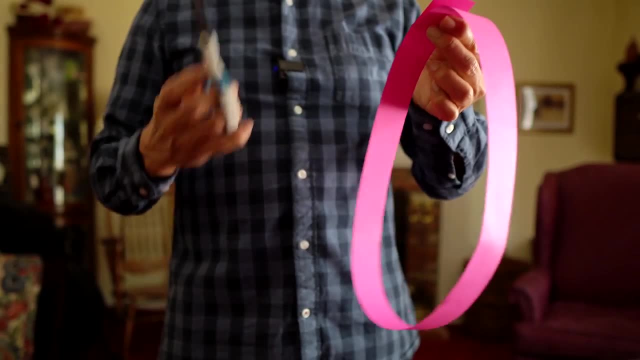 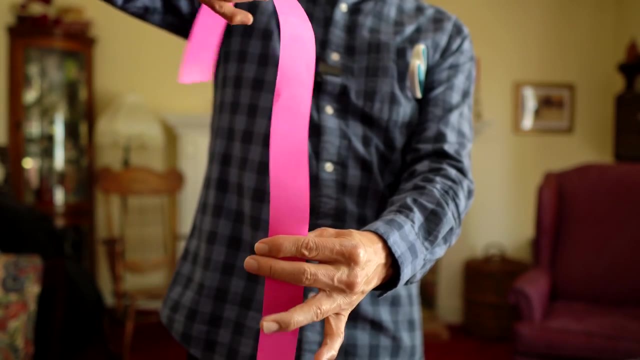 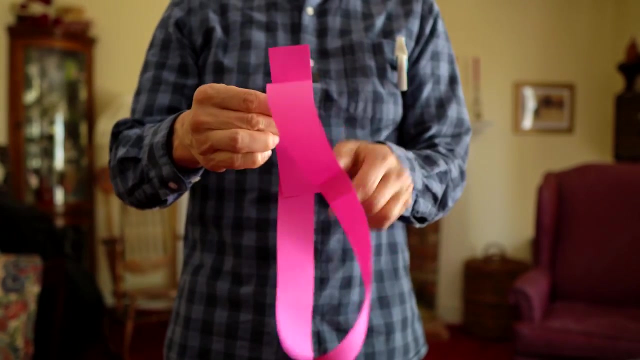 Now the first one, where we made two loops identical loops. all I did was glue these together, Just like this, And this was cut and created the two loops. In the second one you do what's called a half twist, So you take this and you twist it halfway, like that, and then glue these together. 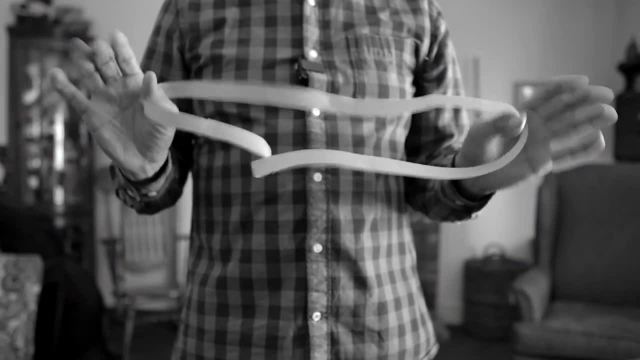 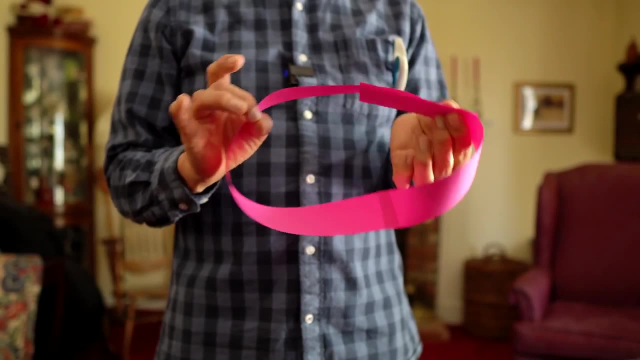 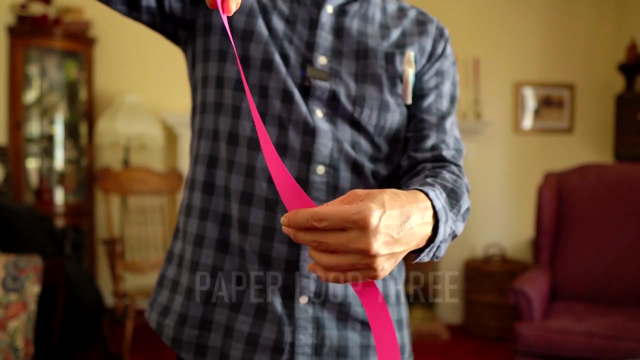 This is the one that creates the loop of interest, the very long loop, and I will talk a little bit about the properties of that which is significant to the scientific angle to this magic trick. And finally, for the last one, where you have two interlinked loops, you twist it a full.